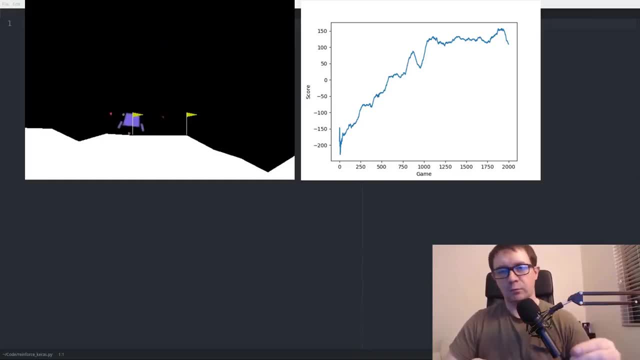 What's up everybody? in today's tutorial, you are going to code up a policy gradient agent. in the Keras tutorial, We're going to tackle the lunar lander environment and, as a bonus, you're going to get to see how to code your own custom Keras loss functions, which is a non-trivial affair. Let's get started. 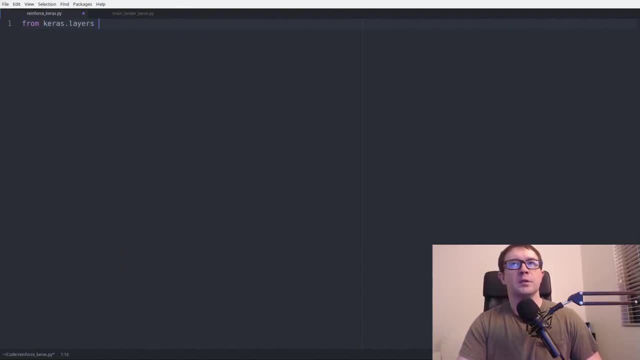 So we start, as usual, with our imports. We want to import our layers which will be dense for the neural network, Activation for an activation function, and input as an input layer. We will also need to import model to construct our model, as well as load model to handle model saving and loading, or loading more specifically. 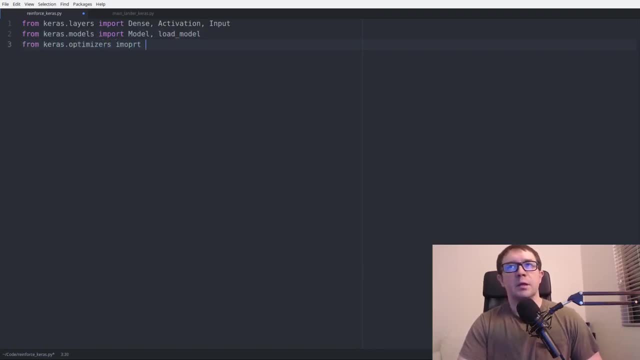 We will also need an optimizer. In this case, we will be using Atom, although you could use stochastic gradient, descent or any other optimizer that you choose. I tend to lean on Atom because it makes life easy. We also need to import the Keras backend. 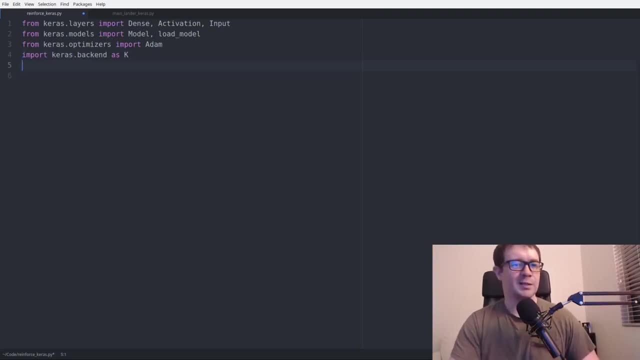 And this gives us access to a bunch of functions that are native to Keras, like clip, as well as log and mean or sum stuff like that. So very important. we want to import numpy as np as usual, and that is, of course, to handle numpy type stuff. 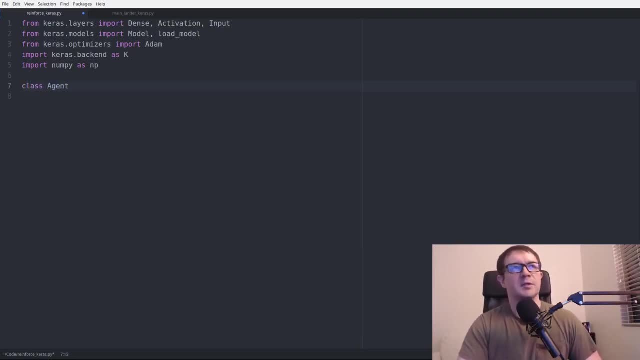 So we are going to stuff virtually everything inside of an agent class And with Keras you don't need to have any specific inheritance from any base Keras classes, like you do with, say, PyTorch. So the first thing we want to pass is a learning rate alpha, a discount factor gamma, if you are not familiar with reinforcement learning. 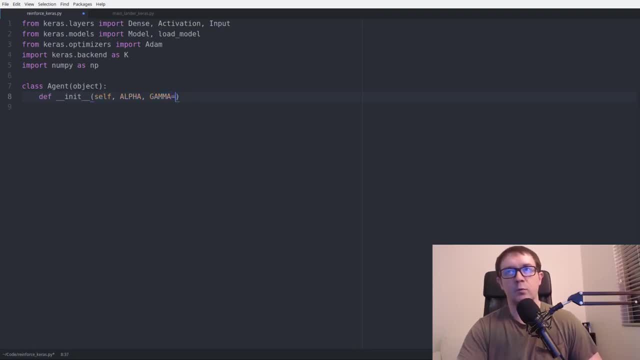 Gamma is how much the agent chooses to discount future rewards, And it is a value bound between 0 and 1, typically something like 0.99 down to 0.95.. For lunar lander, we are going to have 4 actions as our default. 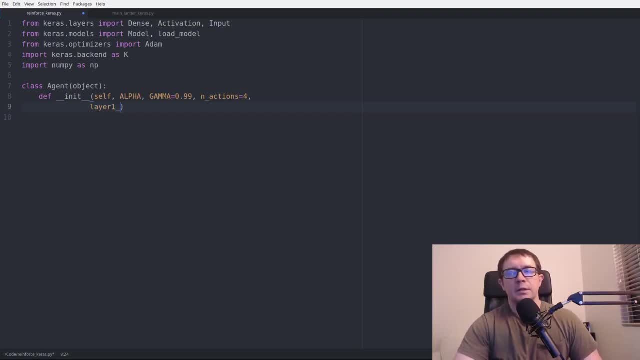 And we are going to have some default sizes for our layers. We will say, I don't know, it doesn't really matter. We will say 16.. Layer 1 size. layer 2 size equals 16.. And input dims will give- I don't know- a default of 128. 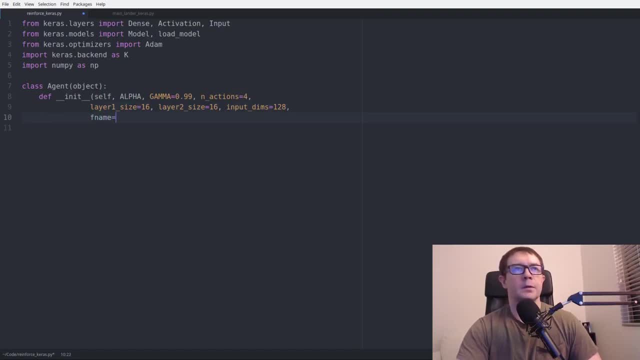 And we also want a file name, something like reinforceh5.. That is to facilitate saving our model- Not so important with the lunar lander because it executes quite quickly, but very important for other more complex environments. So of course you want to save all of your elements. 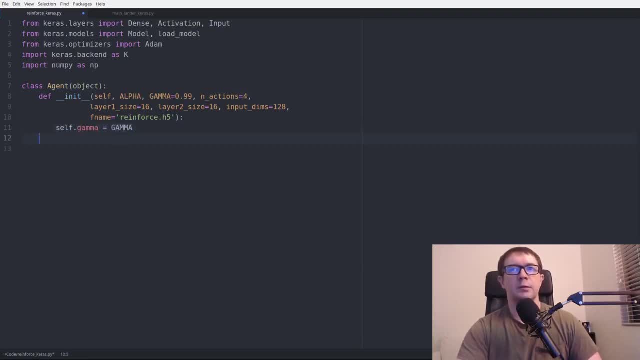 You want to save all of your member variables in their respective fields- Learning rate- we are going to need something called g. G will be the discounted sum of rewards that follow each time step. We will get to that later, But it basically tells the agent how much reward it received after any given time step. 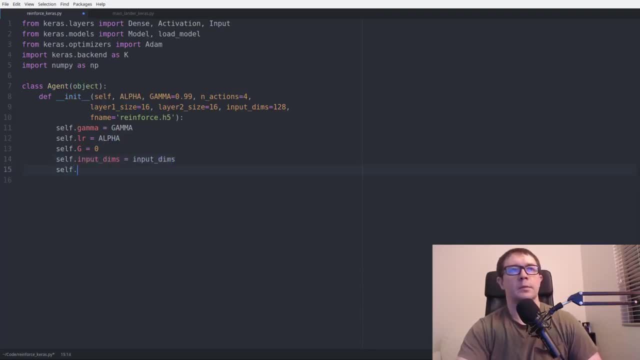 FC1 dims And FC2 dims And FC2 dims Layer 2 size. We also need an actions And this is of course for our action selection. The policy gradient agent does have a type of memory. We are going to handle these as three separate lists. 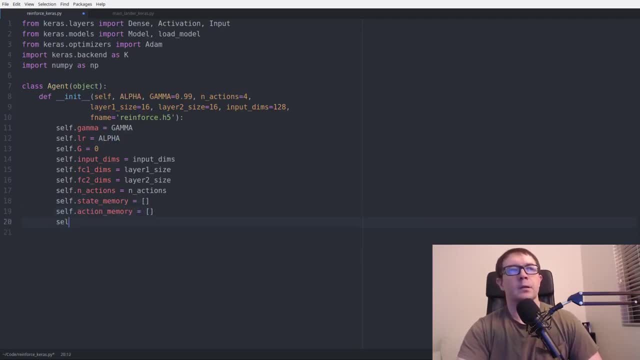 We don't really worry about resulting states in this particular algorithm, like we do with, say, Q-learning, And these are going to get cleared out at the end of every episode, because this is a Monte Carlo method, meaning it doesn't learn with each time step. 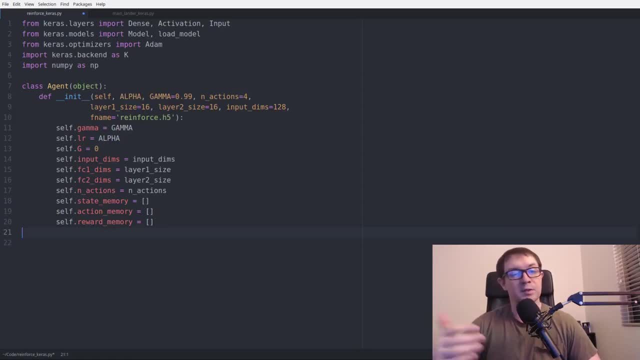 which would be temporal difference, learning like Q-learning. This is Monte Carlo that learns at the end of every episode and we are going to discard all of the memories Now. we could do a batch of episodes- and some people do this- and you probably would get better results with this environment if you did. 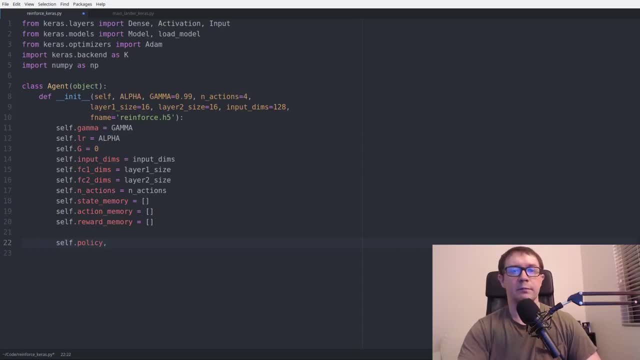 But just for now, we are going to do a single set of episodes. We are going to do a single set of episodes as our batch, So we will need a policy, which is, of course, the agent's probability of choosing any given action, given it is in some state S. 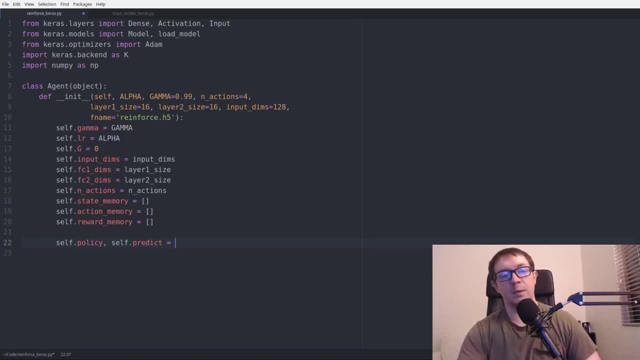 It is a probability distribution. It is what we are attempting to approximate by our deep neural network And predict will be a separate function that we will use to select actions. We need two separate functions because the calculation of the loss requires something called the advantages. 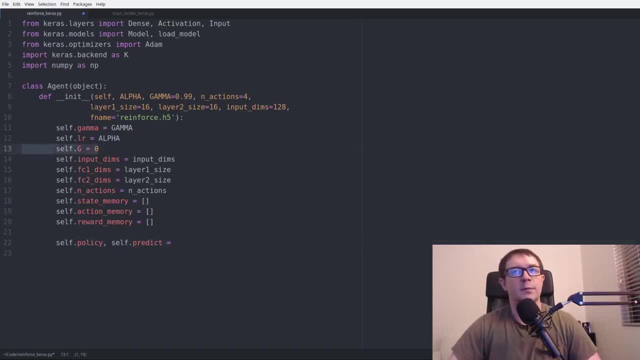 which are just the rewards. It is related to this quantity G up here. It is related to this quantity G up here, Whereas the predict function doesn't need that, It just needs a current state And we will use a function called build policy. 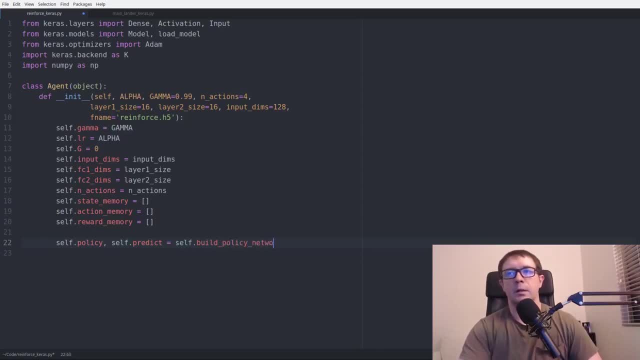 Or say, build policy network, Network that takes alpha and actions and input, dims layer one size, layer two size. I am going to use poor formatting here just for the sake of saving time- And we need an action space That is the set of all available actions for the agent. 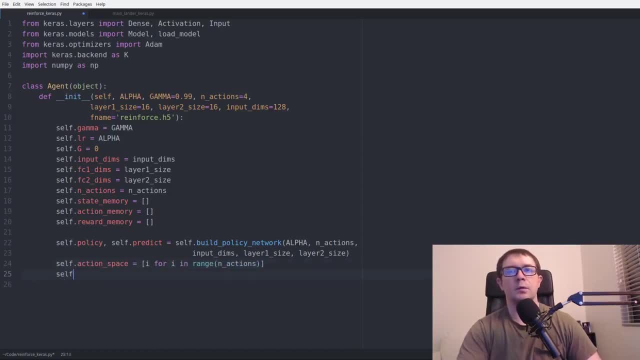 Range and actions, And we will have a model file as well. Okay, So that is our initialize. Let's do our build policy network function. Build policy network That takes in self learning rate and actions. Input dims: L1 size. 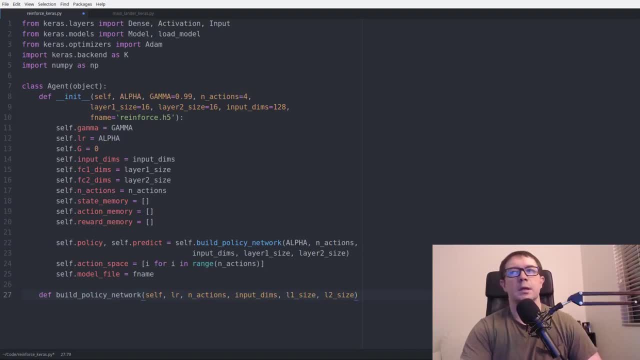 I am going to abbreviate it here- L2 size, And that is it. So we need to declare our input layer That is from Keras, That is the layer we imported at the top And that is takes a shape as input. 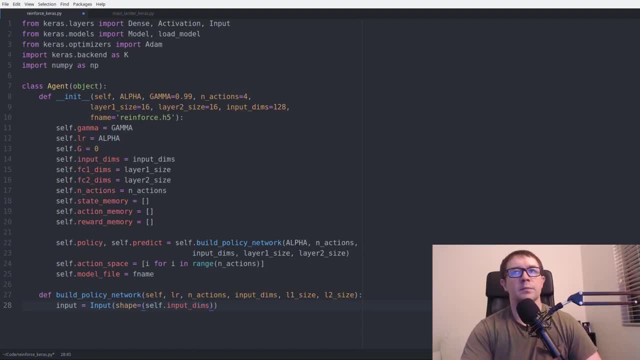 And that must be selfinput: dims comma. That indicates it takes a batch. We also need the first dense layer, Dense selffc1 dims. You know what? Now that I look at it, We don't actually need any of these Because we are referencing self. 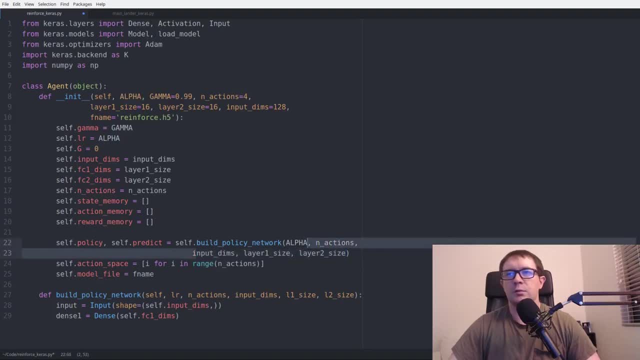 So let's just do this To make things What? To make things nice and neat? So I tend to modify these things on the fly Because, well, you can always improve Right. So selffc1 dims And that acts on input. 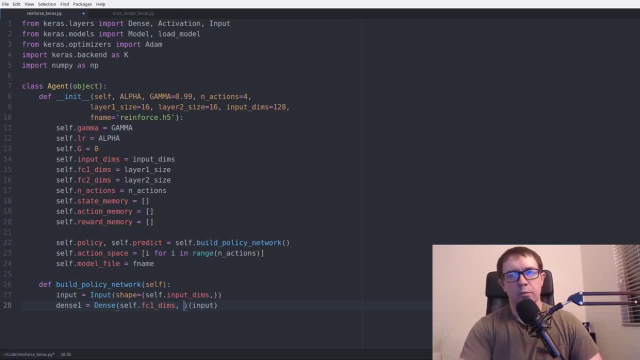 We also have to declare an activation Equals Relu. There is no zero in there, Sorry, And that does indeed act on input. We need layer dense 2.. That is also a dense That takes selffc2 dims Activation. 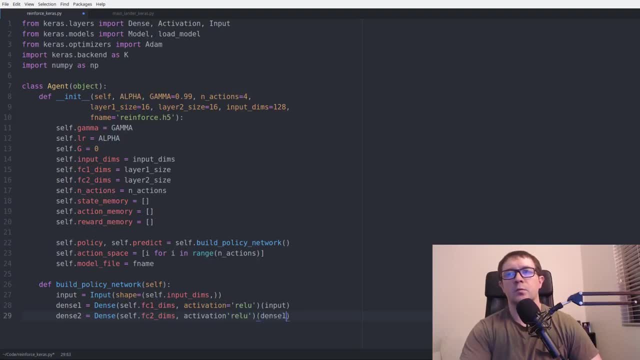 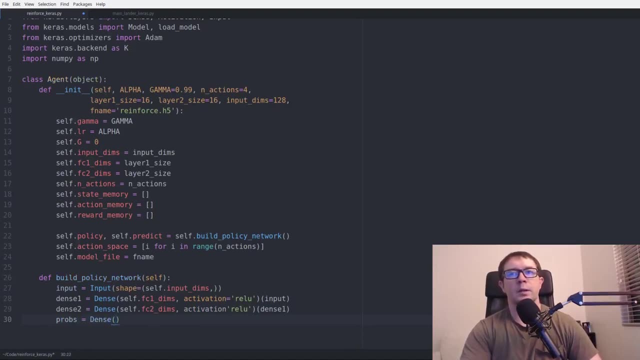 Relu, And that acts on dense 1.. And then finally the probes, The probabilities Equals, a dense layer, And that takes selfinactions as output. We don't specify inputs for the dense layers, Because they are inferred Based upon the input to that layer. 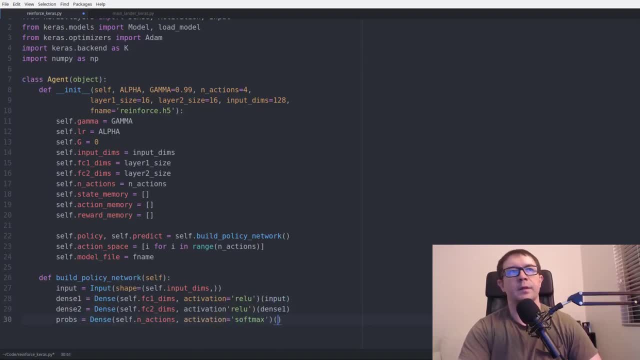 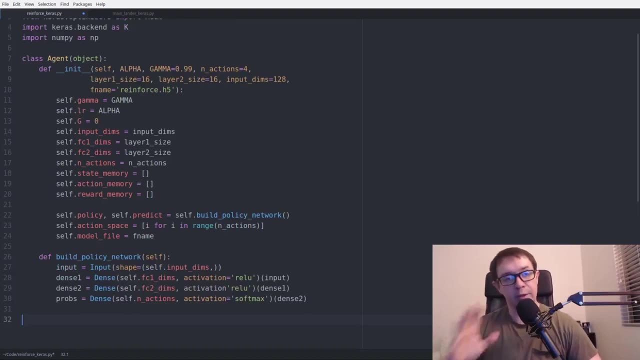 And the activation here is going to be a softmax And that of course, takes dense 2 as input. The reason we want a softmax is because we are calculating a probability distribution And the sum over all, The sum of the probabilities over all possible actions, has to be 1.. 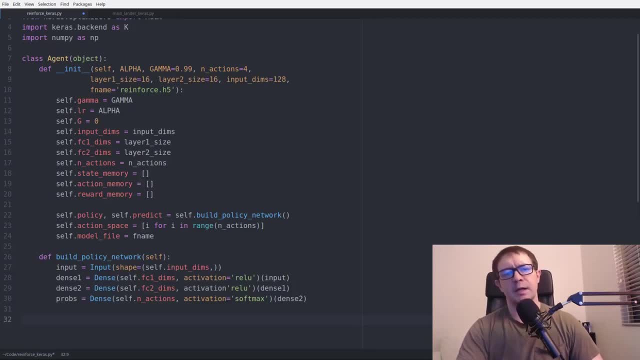 And softmax has that exact property. Now we come to something kind of interesting. So Keras doesn't have an appropriate loss function built in, So we have to write our own. So you do that by using a closure Where you wrap one function inside of another. 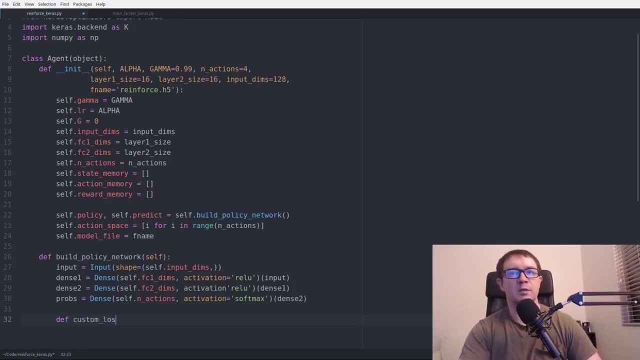 In this case it is going to be two closures. We are going to wrap the custom loss function within the build policy And the reason is that we don't need to access that function anywhere else from the class In the class, So there is no point in putting it as a class function. 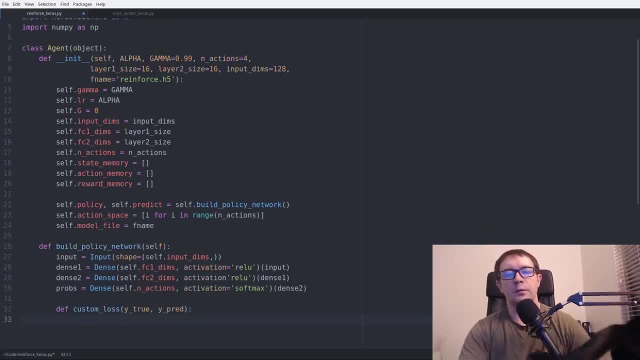 And syntactically, the Keras framework always requires that this has this form: ytrue and ypred. So you must always have that, Otherwise it will complain And out equals K. At least I believe it will. I haven't messed around with it enough to know. 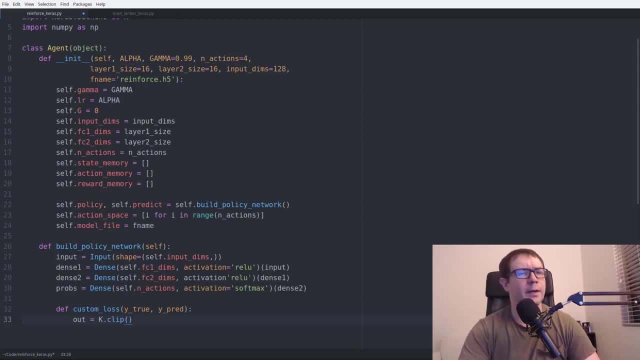 But if I am wrong please correct me in the comments, But my understanding is it has to be ytrue ypred. So since we are going to be dealing with a log Log likelihood, We don't want to be taking the log of 0.. 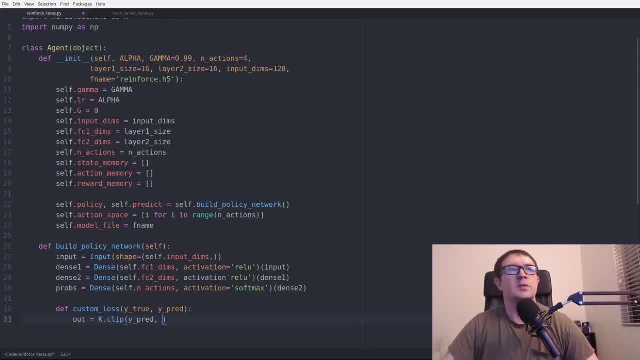 Right, That would be bad. So we are going to use a clip function to clip ypredict Ypredict to a minimum bound of 1 by 10 to the minus 8.. And a maximum bound of 1 minus 1 by 10 to the minus 8.. 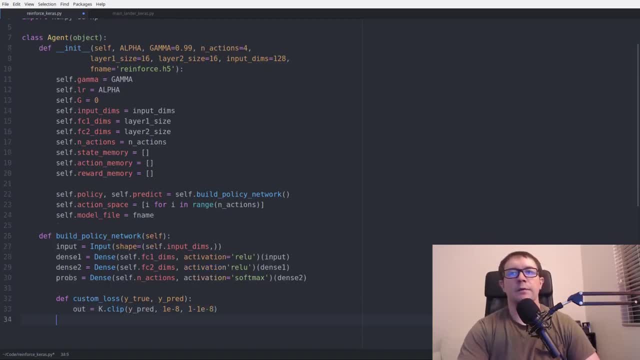 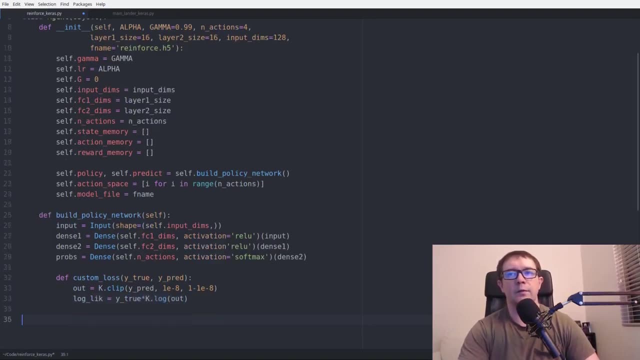 The minus 8.. Yes, And then we will do our log likelihood, That is ytrue multiplied by klog of output. And then we want to return another Keras function: Ksum, minus log likelihood times, advantages. So advantages is something else we have to pass in. 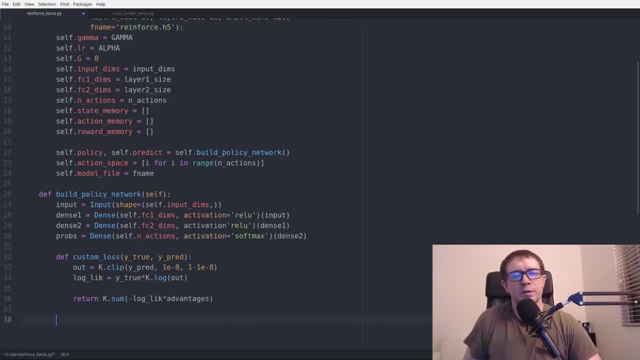 We will get to that in one second. So here this is a double closure. We are enclosing one function. I guess it is only a single closure. We are using one function to return another, And these are all scoped within the build policy network function. 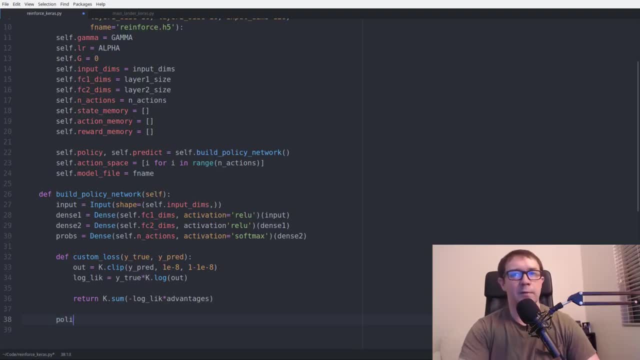 So pretty handy stuff. That is how you handle the custom loss functions in Keras. So policy equals model. Let's see. And the input is a list of input and advantages. Advantages are what we are going to calculate using this G up here. 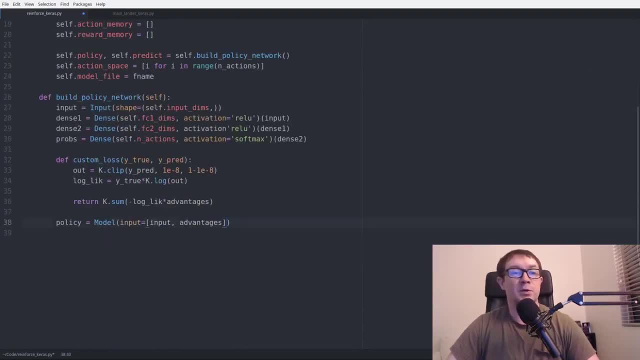 We will get to that in a little bit. But the advantages tell us the reward that followed taking a particular action at a given time step. So it kind of tells you how much reward or what is the advantage of any particular action. And the output of the model is just the variable props. 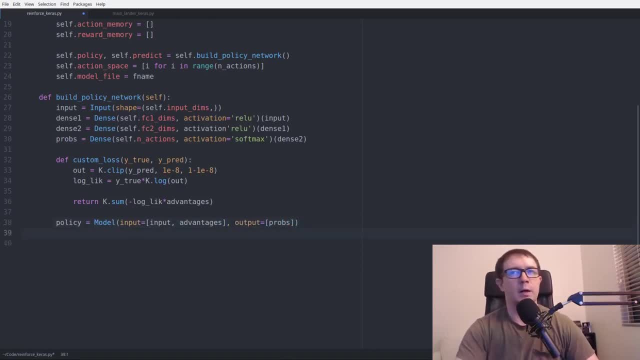 So that connects the inputs and all the layers within the model. Then we have to do policycompile Optimizer. Optimizer equals Adam with a learning rate of self dot learning rate And the loss is custom loss. You don't want to use the parentheses here. 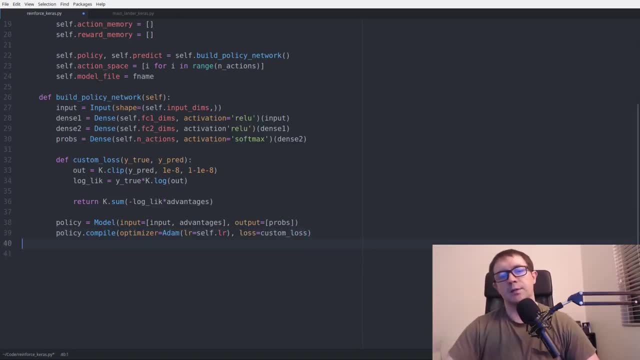 Otherwise it will expect arguments. It is just custom loss as a variable instead of a function, And predict will be a model with input equals, just the input variable or layer rather, And the output will be the probabilities. And we want to return the policy. 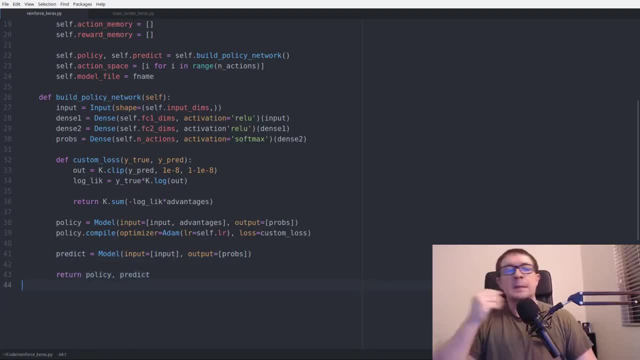 And predict models. So that is really it for the definition of our policy network. Now we get to the more interesting stuff of choosing actions, storing transitions and learning. So let's start with choosing an action And that takes an observation as input. 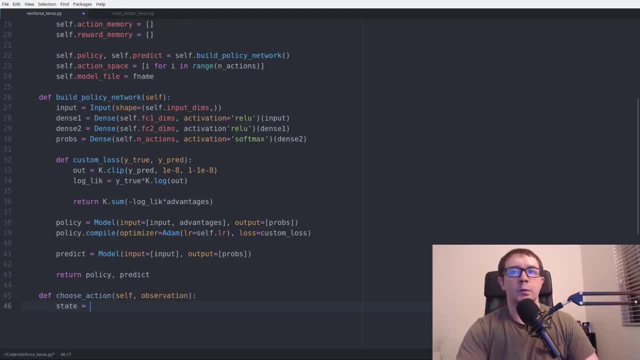 Of course, observation is passed in from the environment. So we want to do a recast, We want to reshape the array, So using numpy, new axis, comma, everything good grief. And what that will do is it will add in a batch dimension along the first axis. 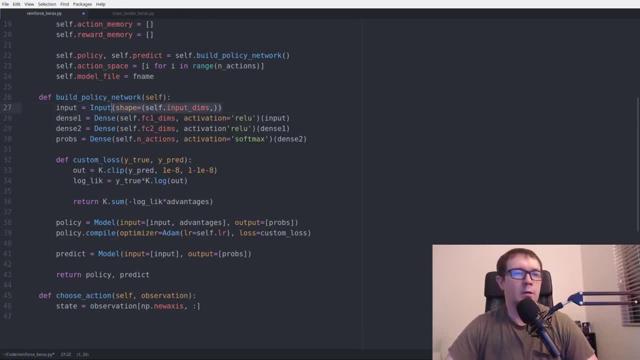 And that kind of allows it makes it line up with this here. That is because when we are doing the learning function, we are going to be passing in a batch The whole state memory of the episode, Whereas when we are selecting an action, we only want to pass in a single observation. 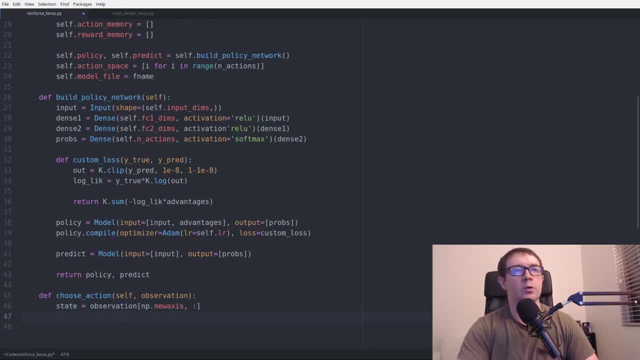 So you have to keep the shapes consistent, So you have to do the addition of the new axis, So probabilities will be self dot, predict, dot predict. Kind of redundant there. Pass in the state and take the zeroth element, because it returns a tuple. 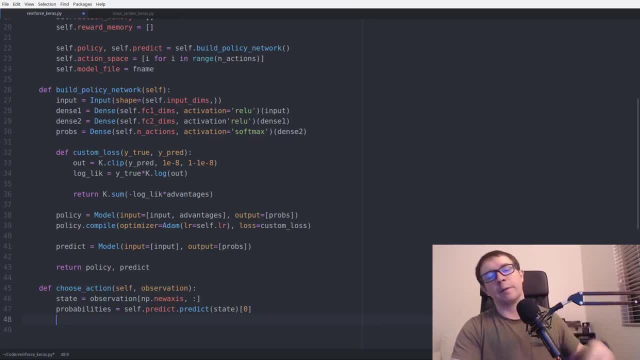 And this is the output of our model. It tells us the probability of selecting each of the actions given. we are in some state s And of course they sorry, in some state state And of course they have to sum up to one per the softmax function. 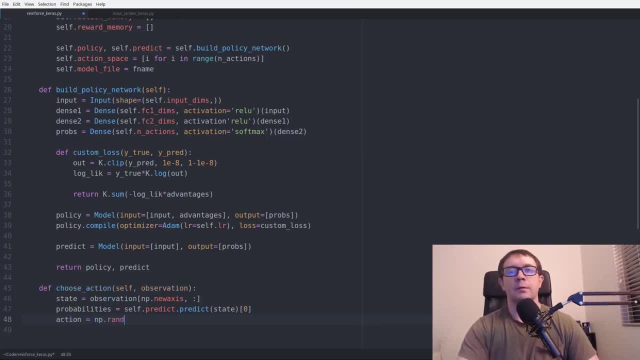 As well as basic definitions of probabilities. Right, The random dot choice. self dot action space. If you didn't know you could do this: You can specify the probabilities for the random choice in NumPy, And that is precisely what we are doing here. 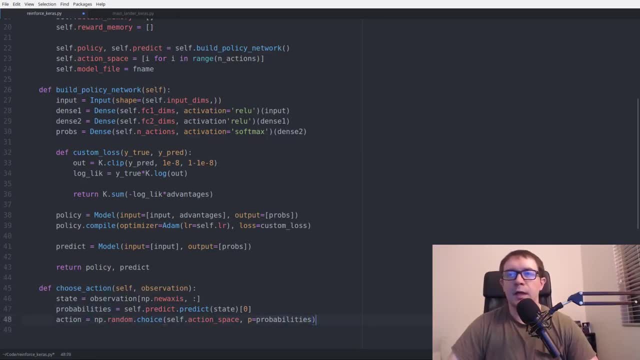 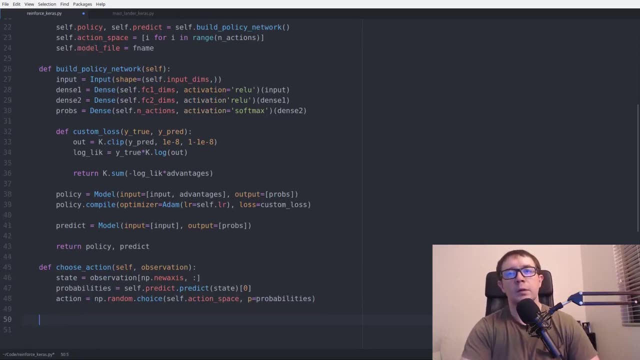 We are using our policy to calculate the probabilities And saying, hey, NumPy, do a random action specified by the probability distribution that we calculate, Very, very cool. And then at the end you want to return the action. Okay, that is pretty straight forward. 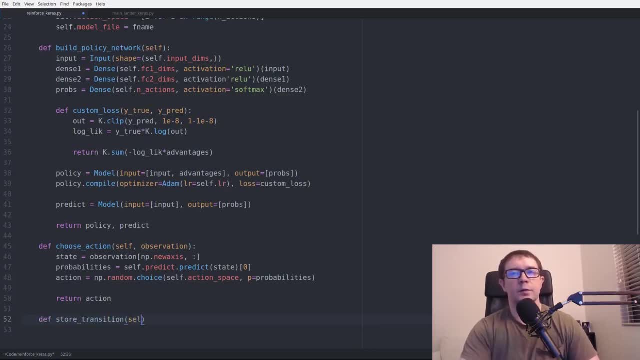 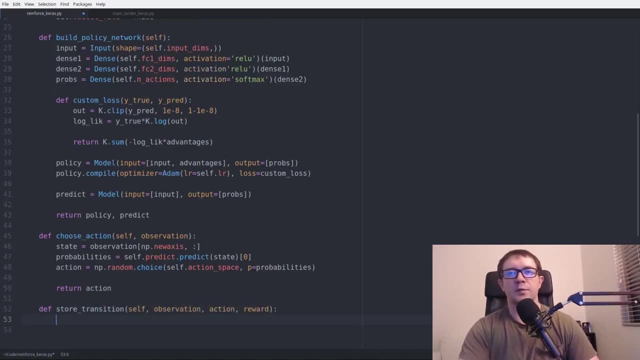 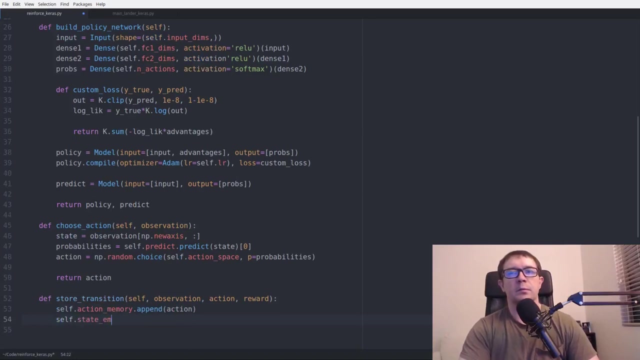 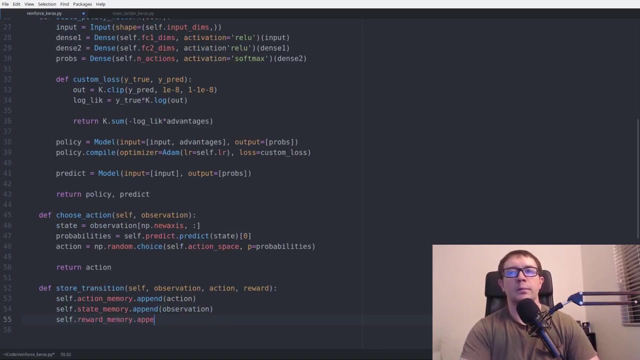 So next let's handle something else. pretty straight forward: Self observation, ervation action and reward. This handles the interface with the memory: Self dot action, memory dot append action, Self dot state, memory dot append observation And self dot reward- memory dot- append reward. 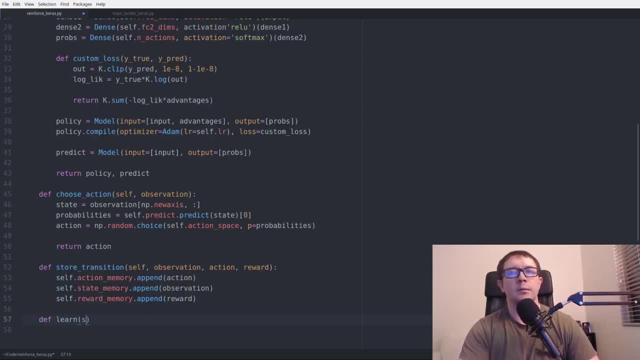 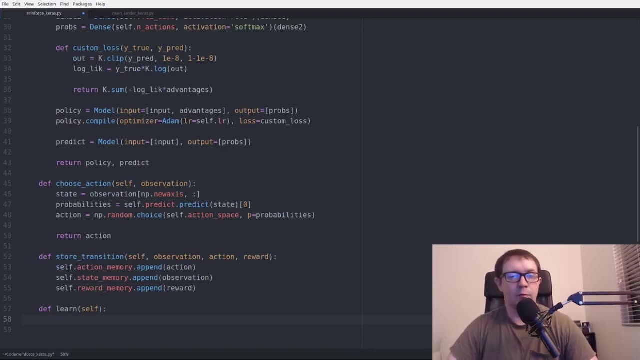 Very straight forward. Now we come down to the learning function, And this is where all of the magic happens. So what we are going to do here is we are going to iterate over our memory of the episode And calculate the returns that follow each time step. 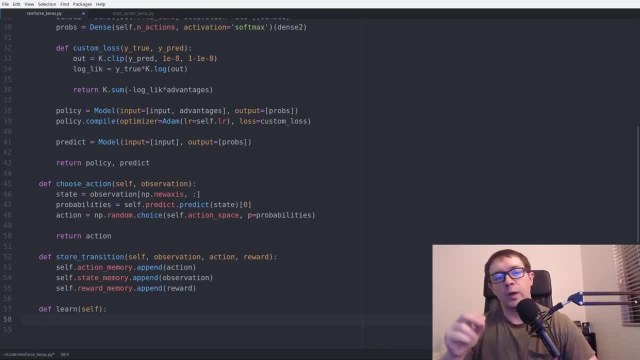 Those returns tell us the advantages or the weights to weight our log likelihood probabilities in our cost function. The reason we do that is because we want to tilt the probabilities in the direction of the actions that give us the most advantageous actions. Makes sense, right. 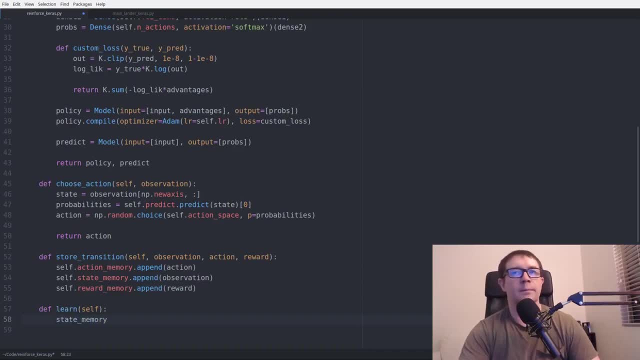 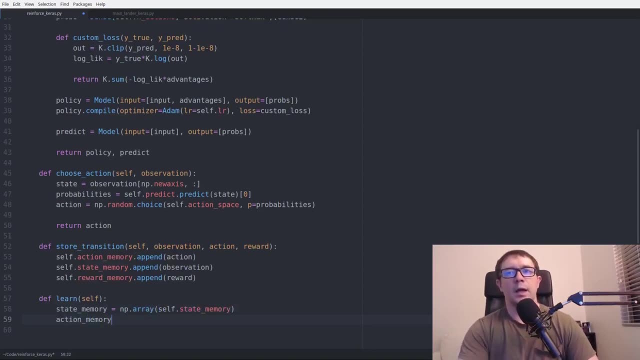 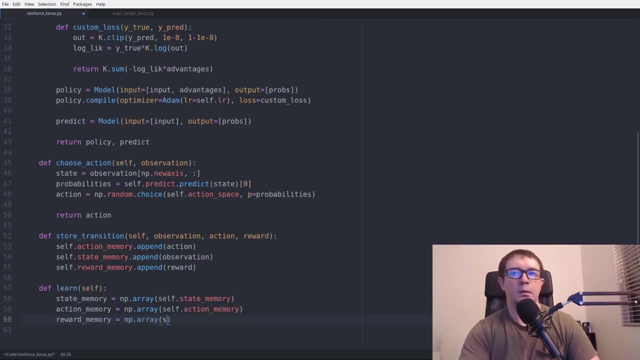 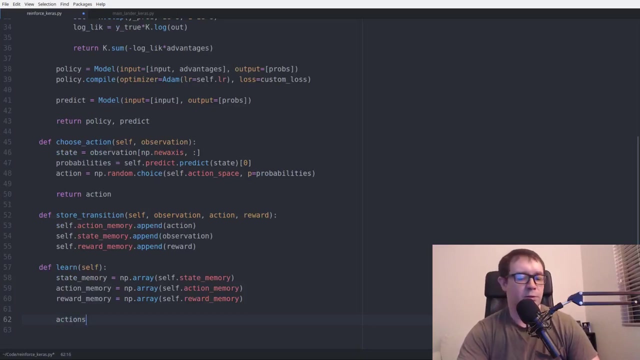 So let's, Let's do this. State memory equals numpy array, self dot state memory. We are just going to turn it into a numpy array to make life easy. Action memory, numpy array, self dot action memory- Perfect. Next we have to take the actions and turn them into a one hot encoding. 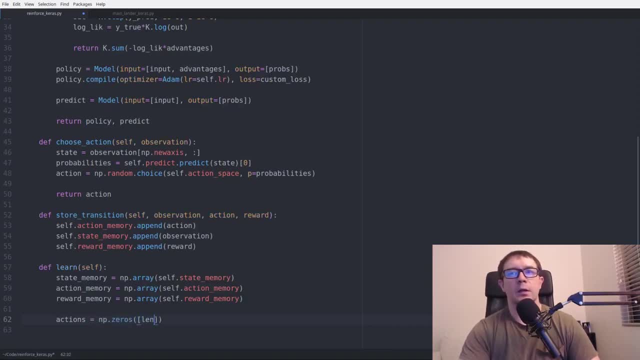 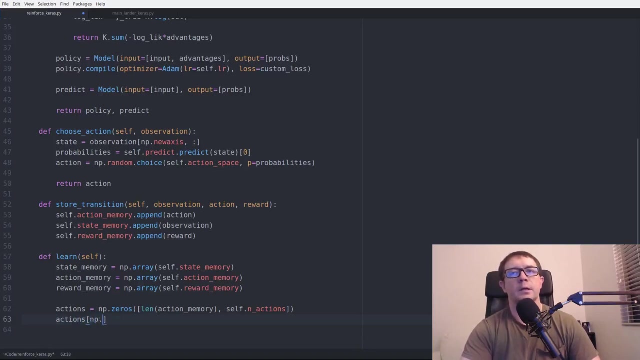 So we can do that, like so Numpy zeros, Len action memory And comma self dot n actions. So yeah, Length of memory by number of actions And then say actions sub mp, dot, a range That gives us the indices Len of action memory. 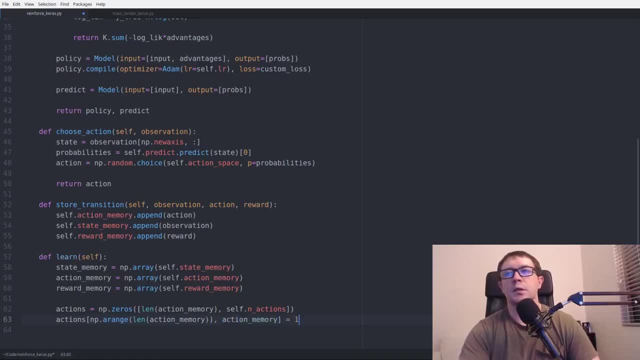 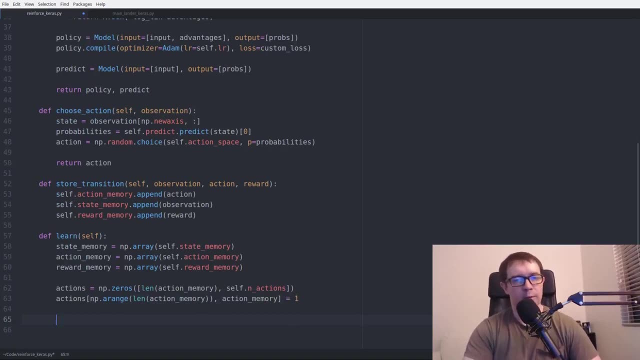 Comma action memory tells us the indices equals one, So that will give us a one hot encoding. And that is necessary for passing in the labels to the loss function, Because it requires the labels to be one hot encoded. So now we can calculate the rewards that follow each time step. 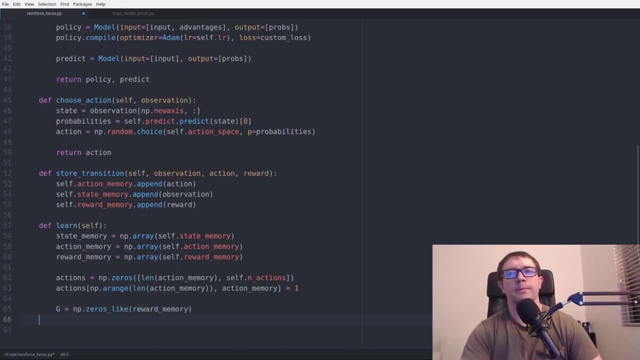 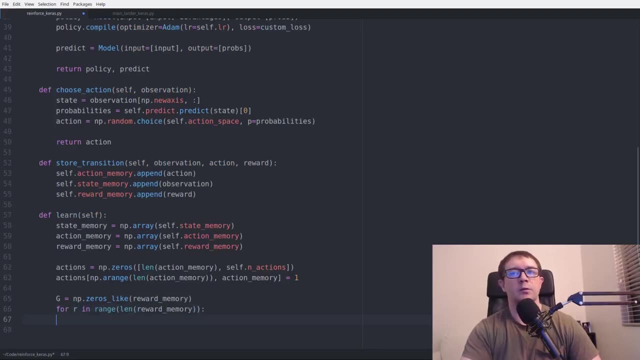 Zeros like Reward memory. Excuse me For t in range Len reward memory. So we are going to iterate over our- Let's call this t instead of r. We are going to And iterate over our memory And calculate what is called the sum. 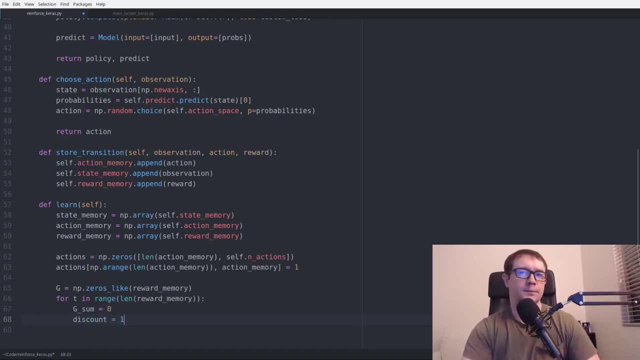 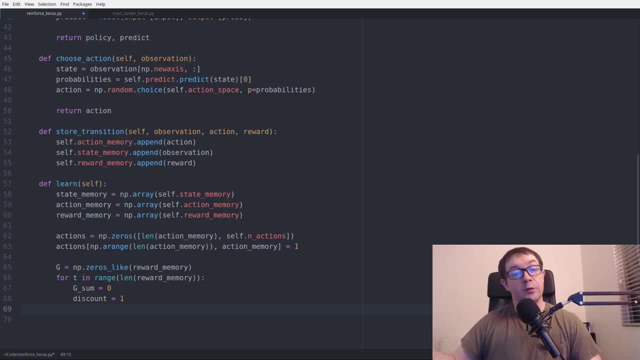 That is the sum of the rewards that follow each time step. We have to take into account the discount factor Because we want to discount rewards that follow each time step By a little bit more, And the reason is that our action selection is probabilistic. 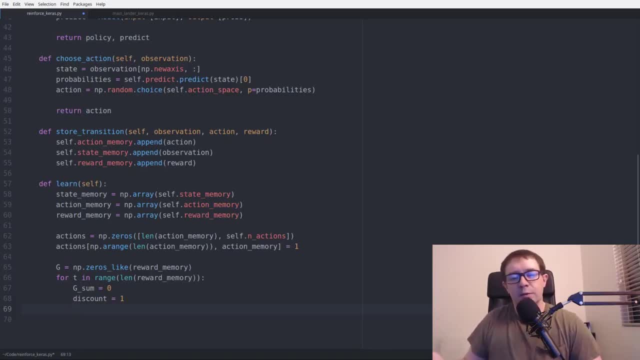 And so we may have chosen that action in this particular instance, But in another we could choose a totally different. You know, in another similar episode we could choose a totally different action, Because we are using a probability distribution And in general those probabilities will always be finite. 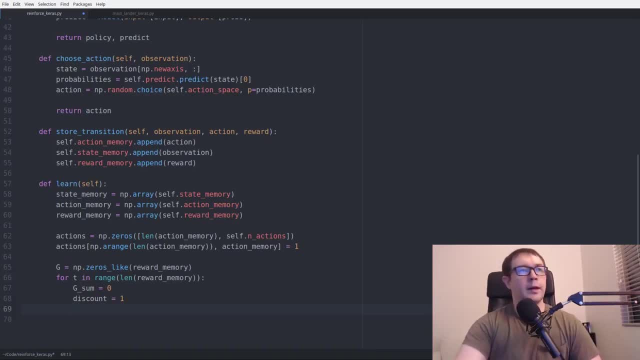 They won't necessarily go to zero. So that is accounted for by the discount factor K in range t. Len of reward memory. So this will start at the teeth time step, Teeth Tooth, Start at the tooth time step And go all the way to the end of the episode. 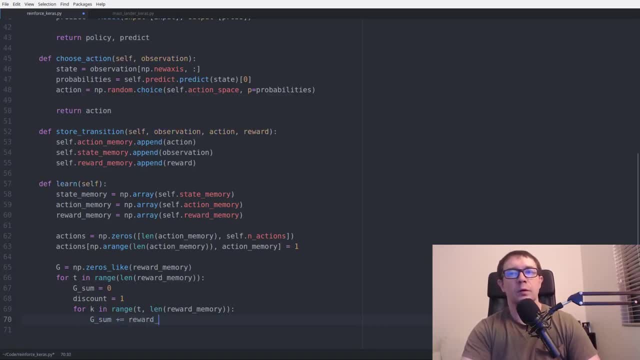 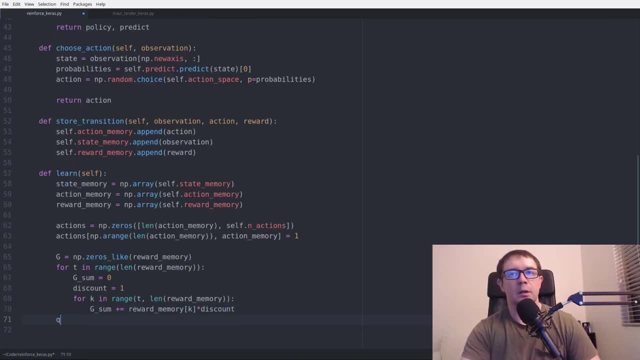 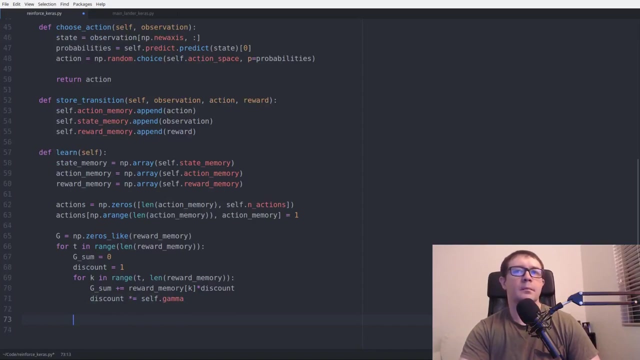 So g sum plus equals reward memory sub k. So this will add the reward Reward at the kth time step Multiplied by the discount factor. And then you want to multiply a discount by self dot gamma In the end of each of those. 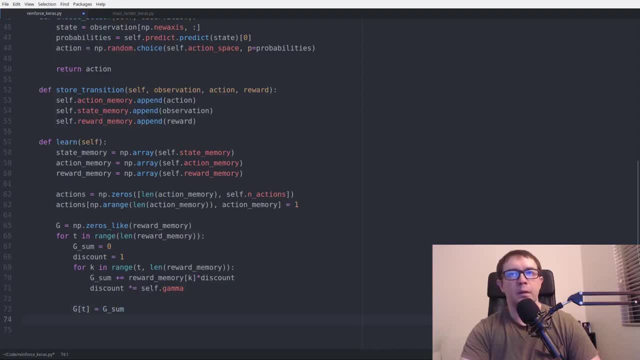 You want to set g sub t equal to g sub sum And at the end of all steps in the episode We want to scale our rewards. This promotes stability Because the rewards in general can have very different, Very different rewards And, as you know, neural networks don't like unscaled inputs. 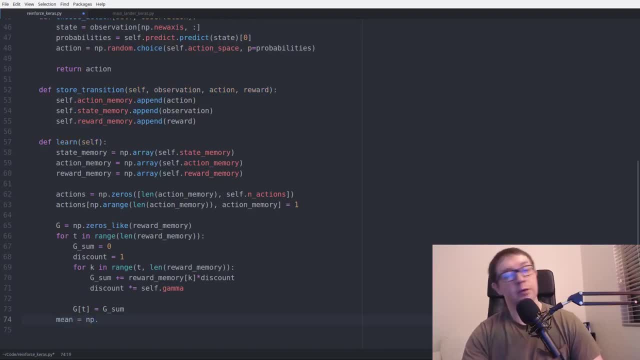 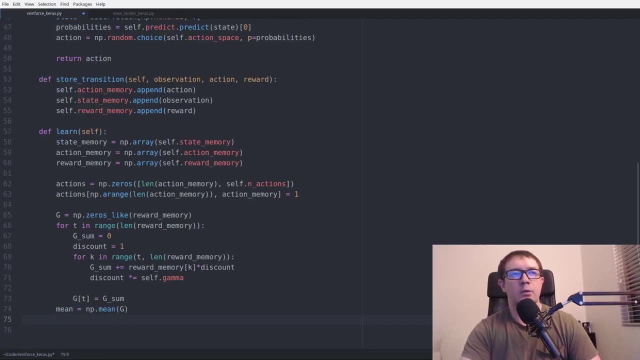 So this is called. This algorithm, by the way, is called reinforced with baseline. So this is the baseline, The mean And standard deviation. mp, dot, mean g And the standard deviation is the standard deviation of g If g is greater than zero. 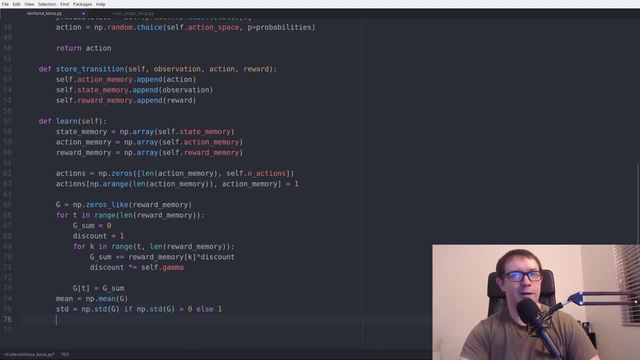 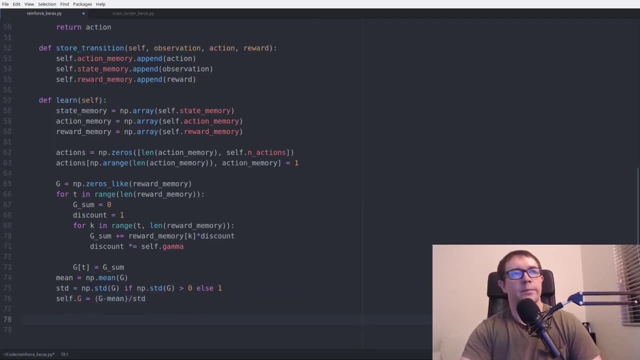 Else one, Because the standard deviation could be zero. You don't want to divide by zero, Right? Don't cross the streams, That would be bad. So g equals g minus mean Divided by standard deviation. So that handles the calculation of the. 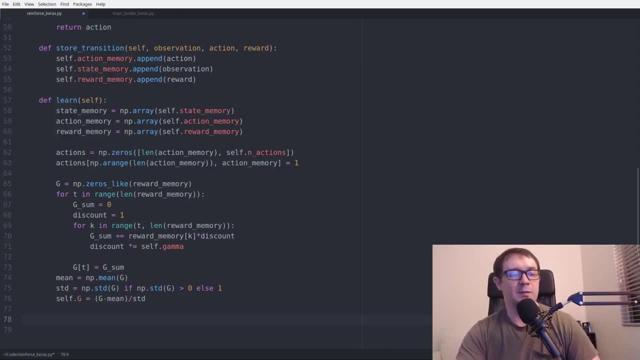 The discounted feature rewards that follow each of the t time steps With our scaling and normalization. So let's say cost equals self dot policy, Dot train on batch And we pass in the state memory- That's our input- As well as self dot g. 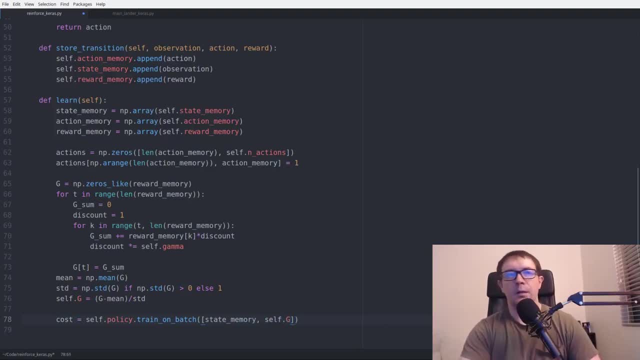 Self dot g is our advantages And we have Actions. I just call it actions So that Those are our actual labels. These, This will be the Why predicted And these will be the why true For our loss function. 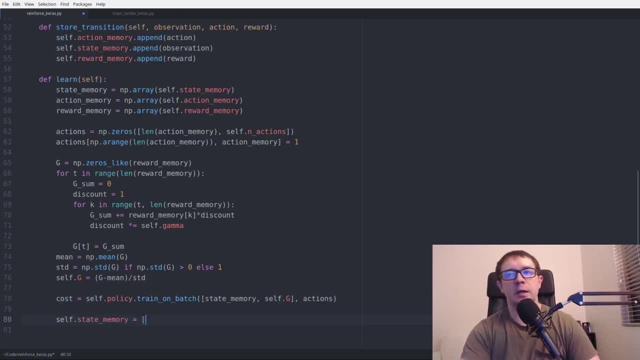 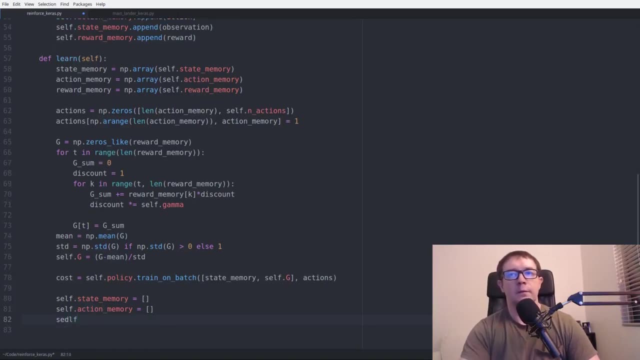 Once that is done, We are done with our memory for the episode, So let's go ahead and reset it. No point in keeping it around. This is, after all, A Monte Carlo method, And Same for the Reared reward memory. 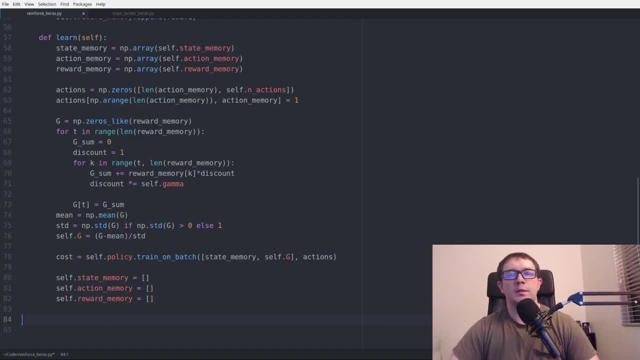 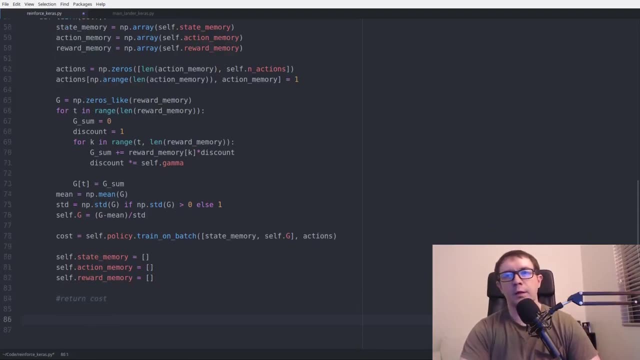 And That is it. If you want, You can return the cost. If you want to kind of plot the cost over time, If you're into that kind of thing, You can do that. Next, We have a state Save model. 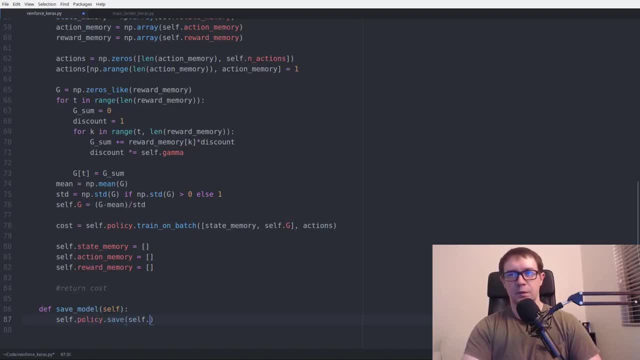 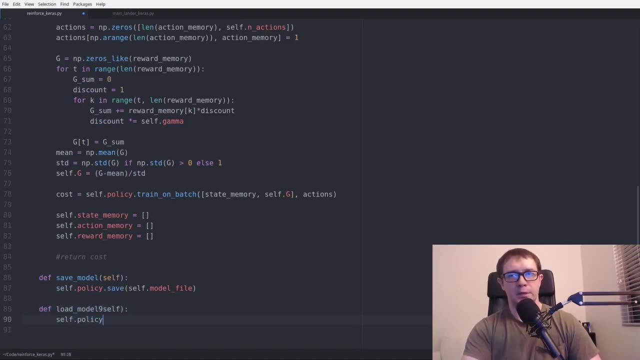 Self dot policy. Save, Excuse me. Self dot model file. Def load model. And Self dot policy Equals Load model. Self dot model File. Of course I'm looking at it Like. the colors are All wrong. 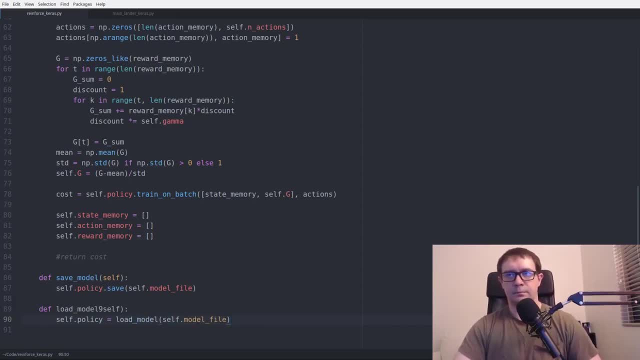 I wonder what I did wrong. I added it In an extra nine. Okay, So This is 90 lines of code Plus some white space Right, Plus minus some white space. So this is a pretty short program And this handles. 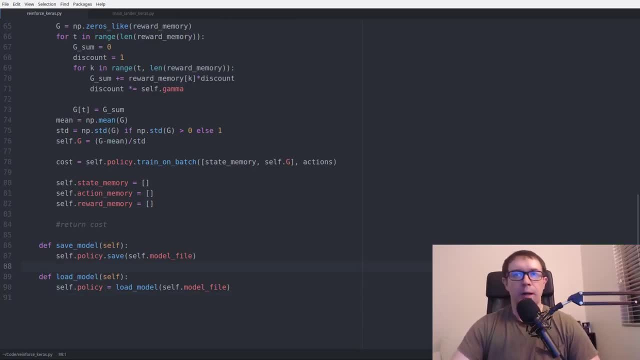 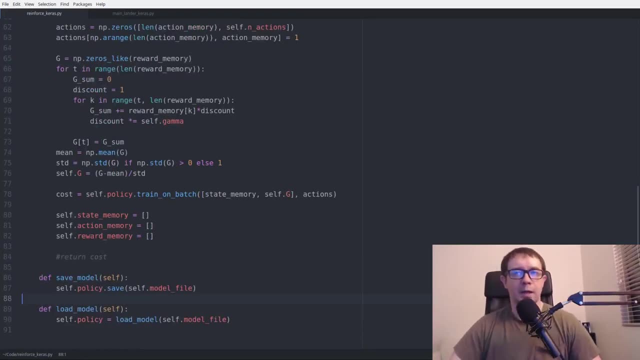 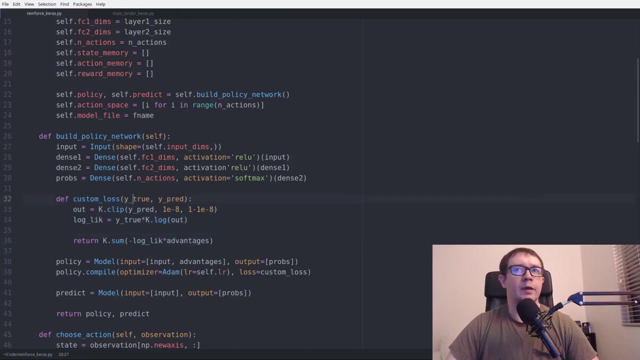 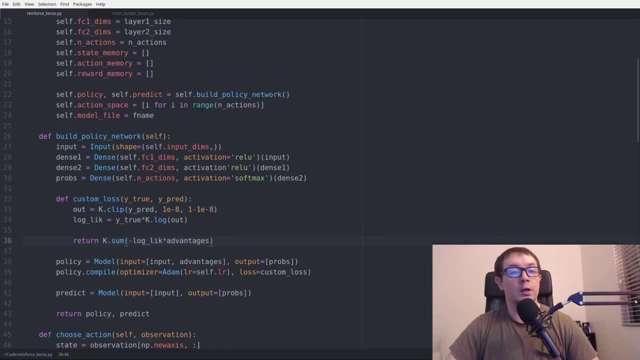 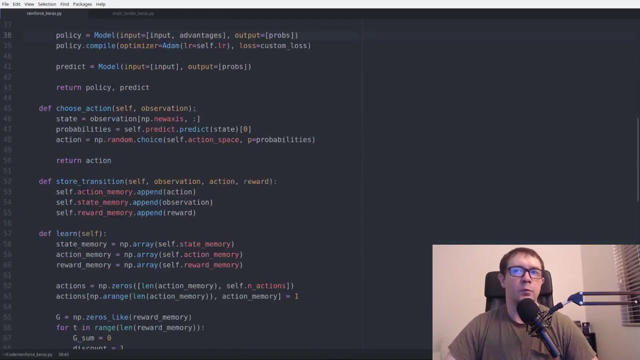 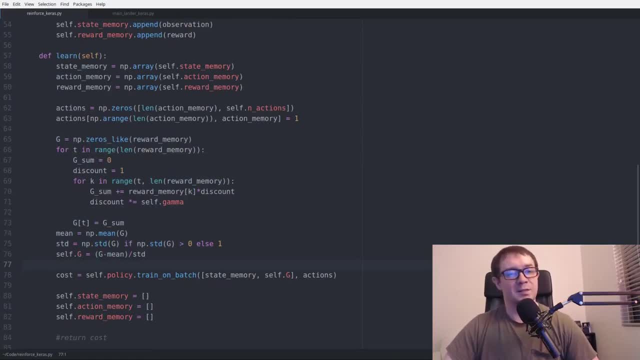 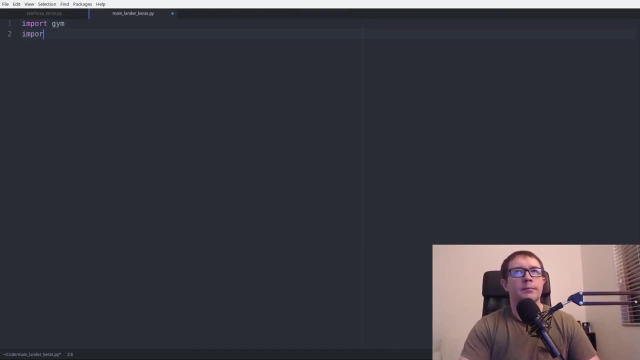 let's head over to the main program and start writing up some code, test this out and see how it does. so we start with our imports. we'll need Jim, we'll need mat plot, live dot, PI plot, SPL, T. we will need num pies and P to take a look at the 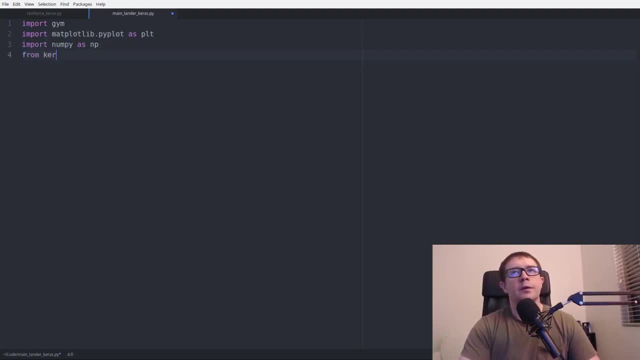 average rewards we will need from reinforce Karas import agent and from utils import plot learning. I'm not going to plot it here. you've already seen the plot at the beginning of the video. we're not going to bother with that again. but that's where you would import it, so the name equals main. then we want agent. 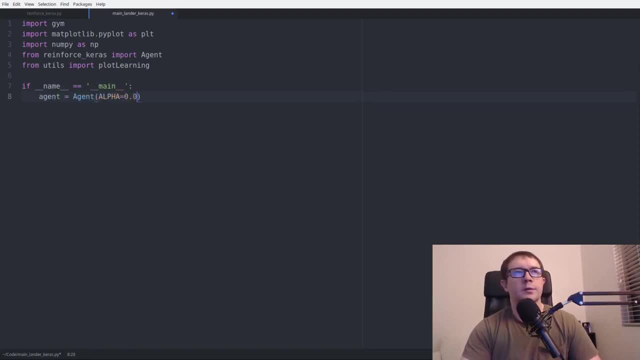 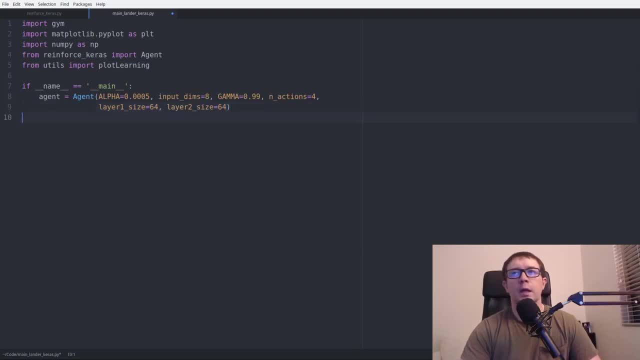 size equals 64, and these are kind of what I found to work. so just a spoiler alert policy, gradient methods and the reinforced algorithm in particular, is a incredibly simple and efficient because we discard all the memories that at the end of each episode, so doesn't make very good use of everything that. 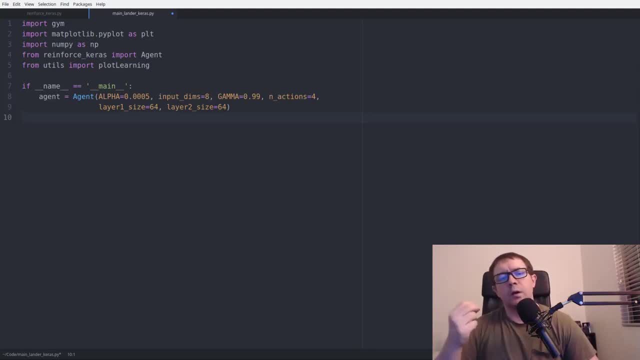 happened prior to this episode. and two, they are incredibly sensitive to perturbations in the change of the parameters. so what that means in practical terms is that, as we do the gradient descent, as we vary the parameters in the neural network very slightly, that results in big changes in 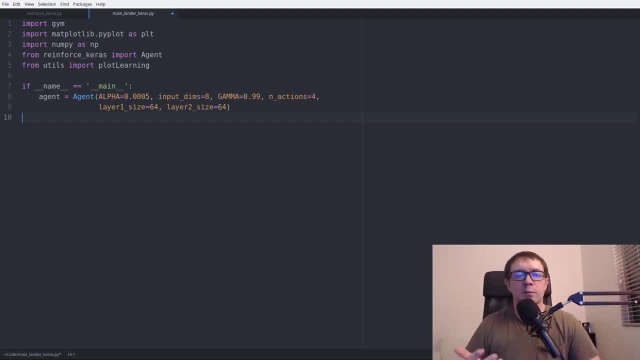 parameter space. really, what we're iterating, what we're navigating here, is parameter space rather than anything like cost space, and so that gives you big changes in the model, and so it is a little bit unstable. I haven't done a whole lot of hybrid parameter tuning. this gets a decent enough result. it doesn't quite beat it I. 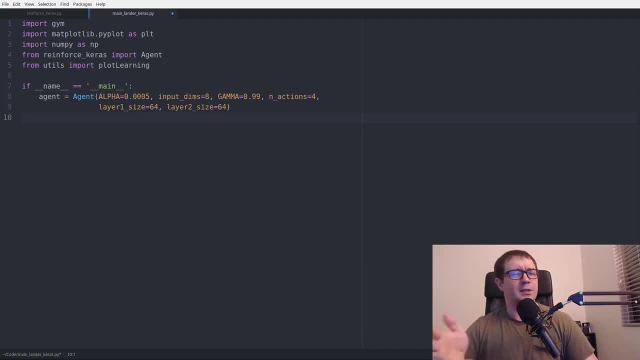 think of my pie torch version. it did beat it. there's always a slight the differences between versions, but now this forms a conceptual basis for other stuff, like actor critic methods and deep deterministic policy gradients, which we've covered here on the channel as well, and we'll do a couple more videos. 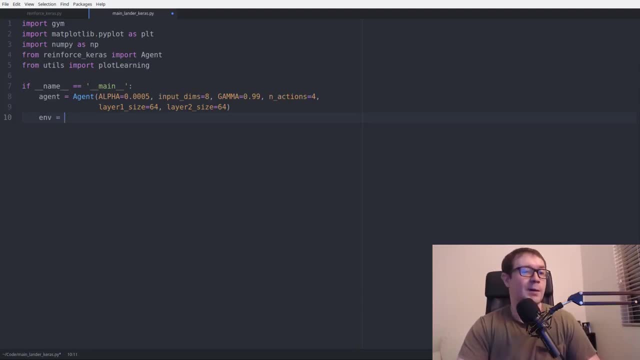 on them in the future. but just keep in mind that, though you do not see the best possible performance, you are free to do so, and I'll see you in the next video. and I'll see you in the next video to go ahead and tweak this on your own time and try to get the best possible. 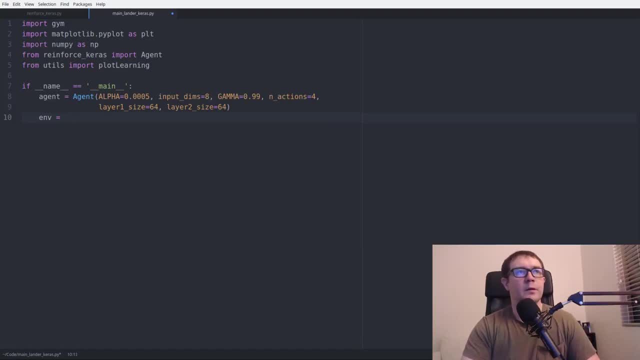 results. I would encourage that and ask you to do that as well. so let's do our environment. lunar lander v2 score history. of course, what we used to keep track of the scores and episodes 2000. the consequence of the sampling efficiency is that it takes far more episodes to converge to something. 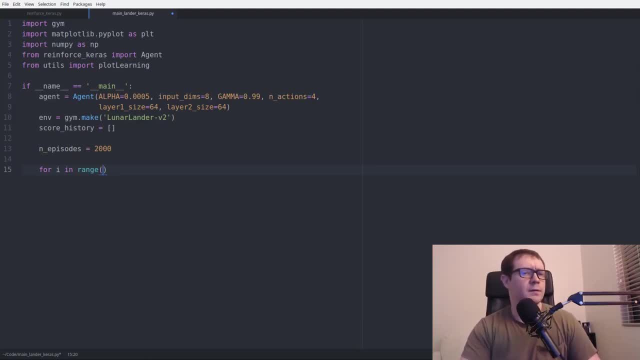 reasonable, whereas in deep Q learning we basically have it solved within 150 to 200 episodes. episodes done equals false, score equals zero. observation equals the env dot set spot done action equals agent dot. choose action observation observation underscore reward. done info equals the enemy step. agent store transaction. 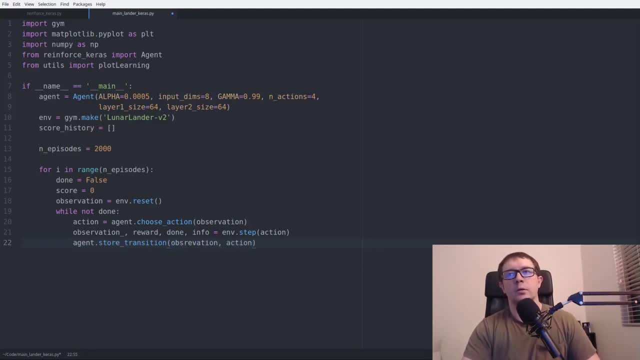 observation: observation action that's misspelled. observation action and reward: observation equals observation underscore score plus equals reward score history dot append. score blank: equals. I don't think in this case I return anything, so it's agent dot learn. 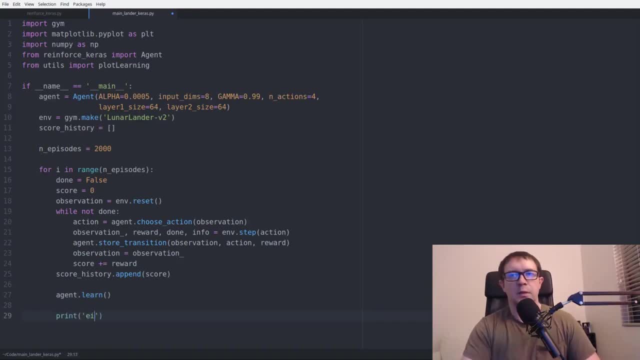 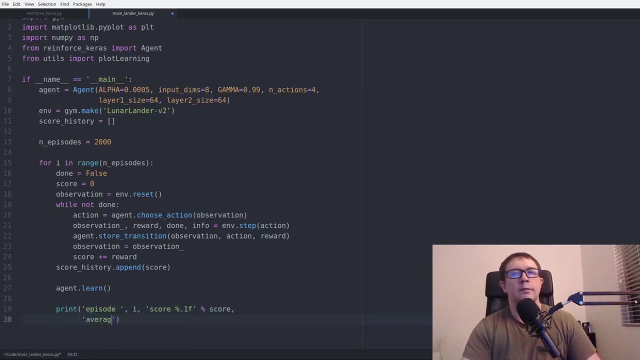 and then we want to say print episode and um come I score. 1F percent score uh, average score percent. 1F percent MP mean score history minus 100, um. 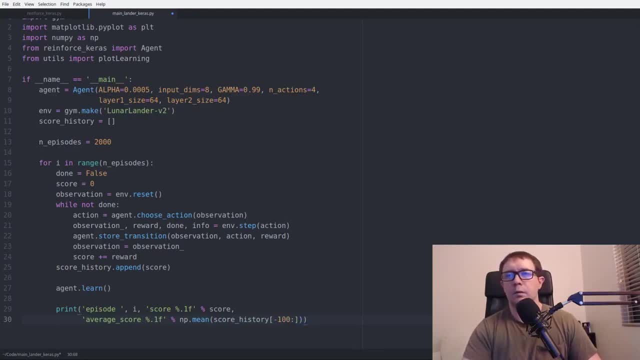 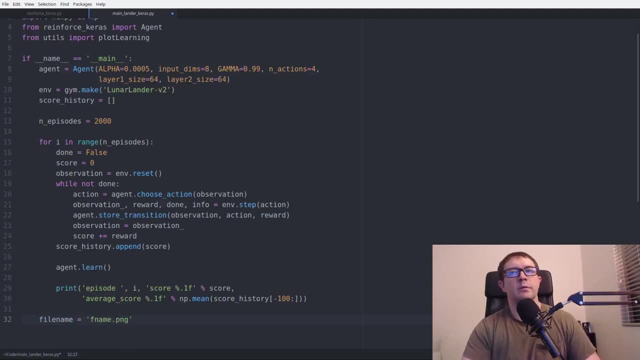 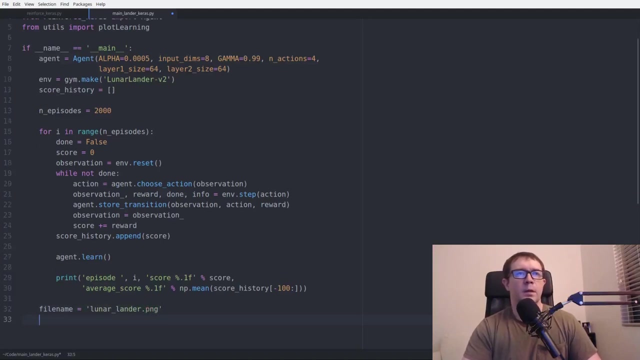 and that is all I want to print. so the end file name equals F name dot PNG, whatever. well, let's call it lunar lander, lunar lander, dot PNG. and plot learning score history. file name equals file name. window equals 100, okay, so that is pretty straightforward. 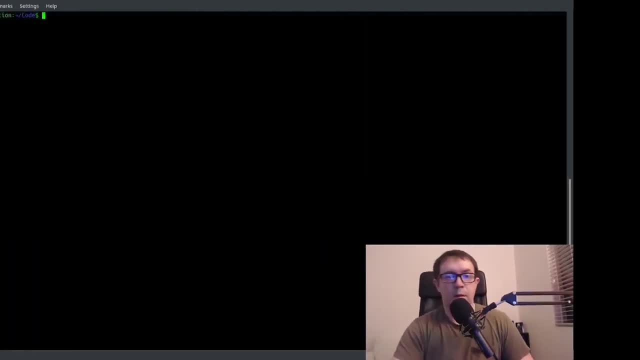 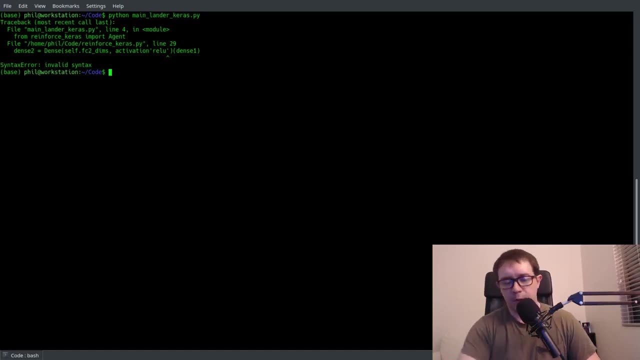 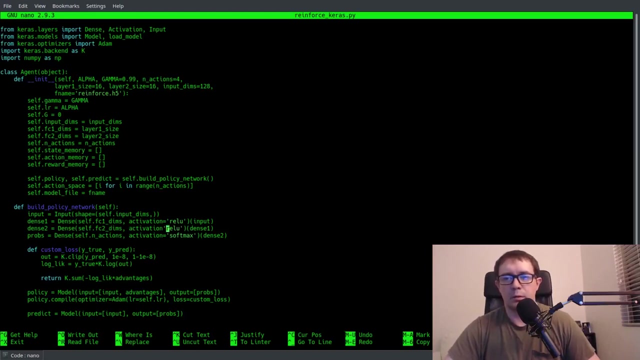 let's head to the terminal and see how many typos I made. all right, python, main lander. okay, I forgot an equal sign. okay, so let's just use nano. that is here. activation equals, and here I have an equal sign. okay, let's try it again. 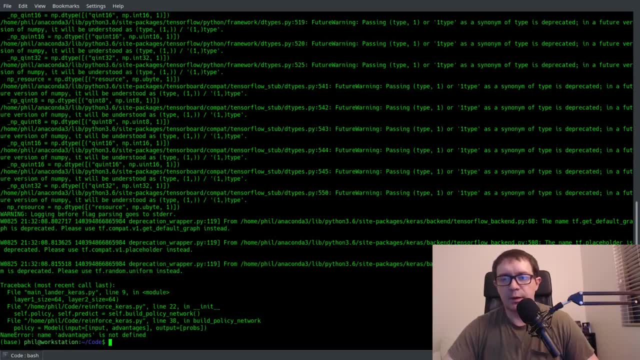 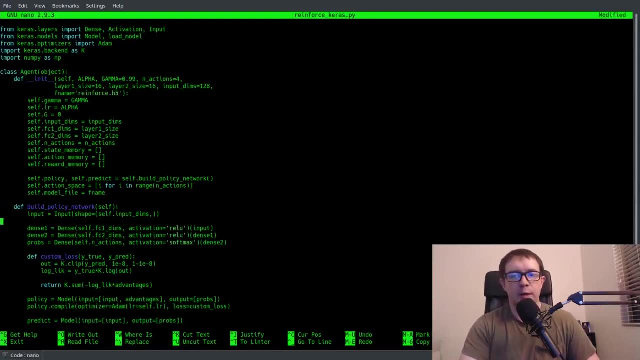 okay, name advantages is not d find. oh, I forgot the input, so that's why that makes sense. you probably were wondering that let's say advantages equals input. uh, shape equals 1, and that is that. let's try it again. 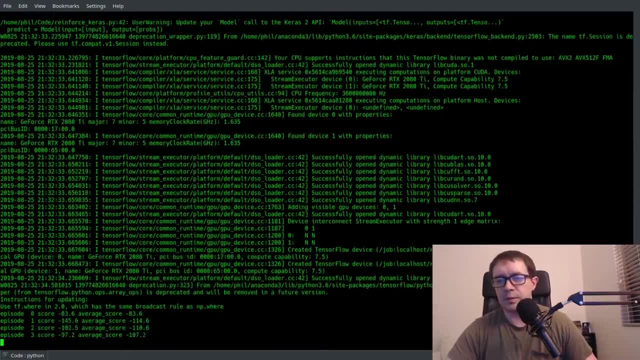 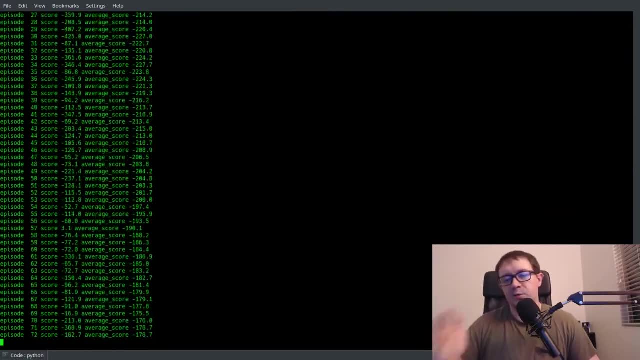 oh, it doesn't complain about nope, it does not complain about the spaces, and it is running. I only made a couple typos, or pretty good, pretty good for old Philly, so okay, so it is running.